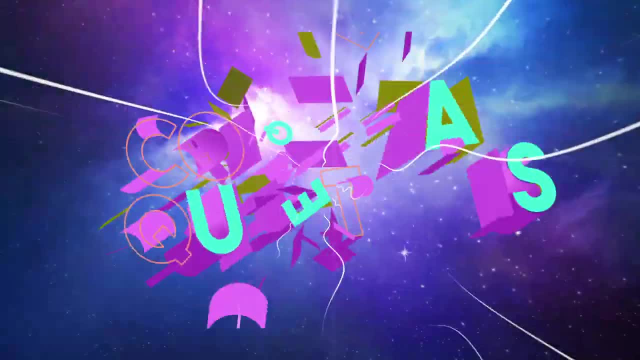 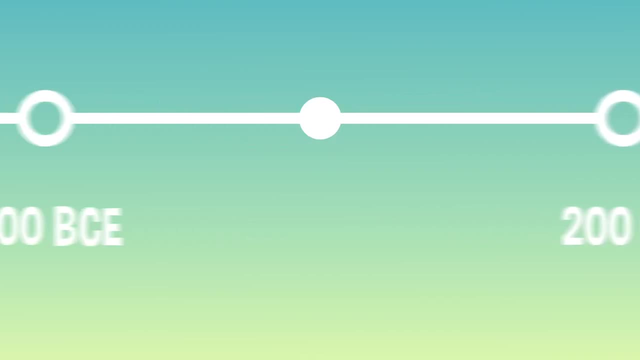 Let's find out on today's episode of Colossal Questions. The very first Olympic Games on record date back thousands of years, to 776 BCE, in a Greek city-state named Elis. And that's just the first games we know about. Most experts believe the Olympics. 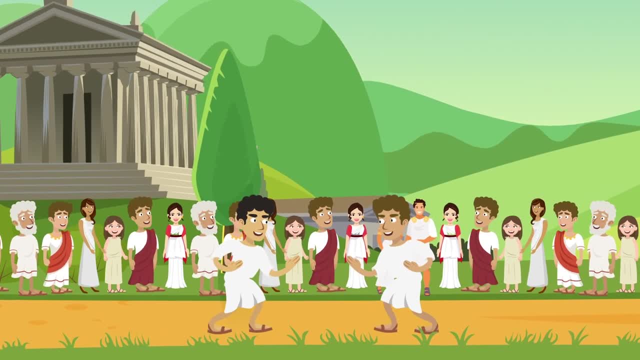 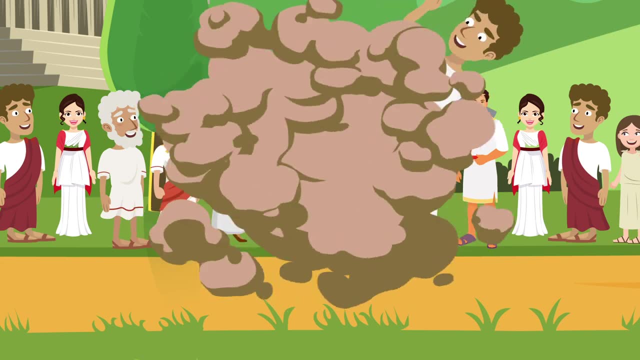 were already 500 years old by then. So, needless to say, it's one of humanity's most ancient athletic competitions, Just like today. the ancient Olympics were held every four years, and athletes were able to compete in the Olympic Games every four years. 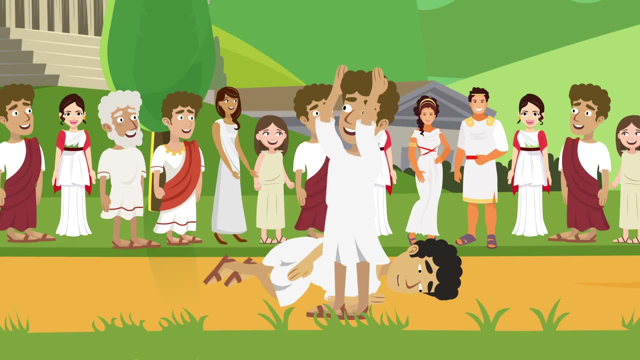 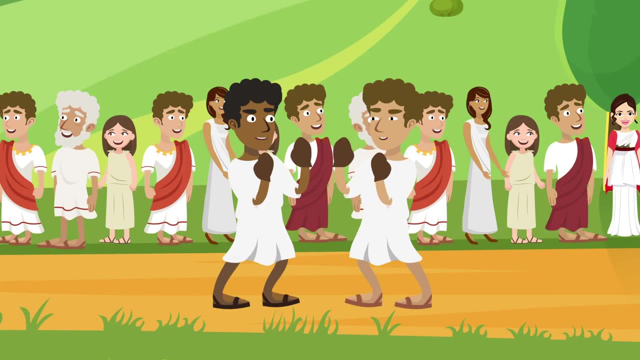 So, needless to say, it's one of humanity's most ancient athletic competitions. Just like today, athletes came from city-states across Greece to compete. Early Olympic Games consisted mainly of foot races and wrestling, But over the years the Greeks added other games like boxing, discus. 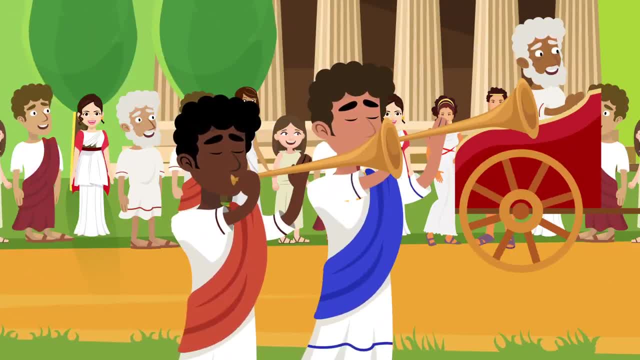 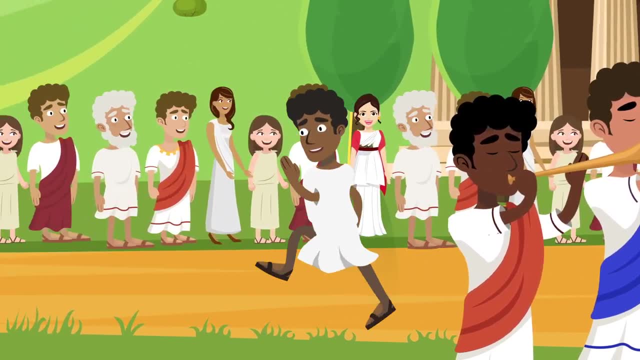 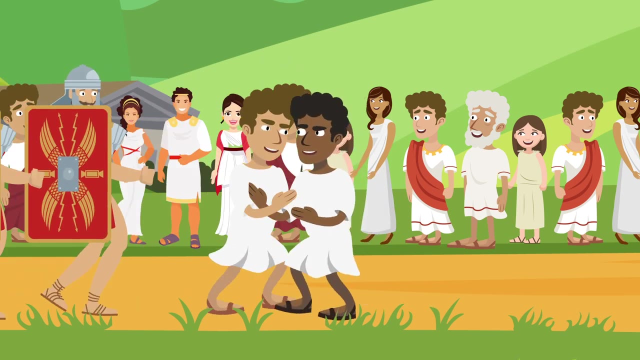 javelin, chariot racing and even competitions for heralds and trumpeters. The more grueling events were often bundled together to create larger contests, like the pentathlon, which includes a foot race, the long jump, discus, javelin and wrestling. With the rise of the Roman, 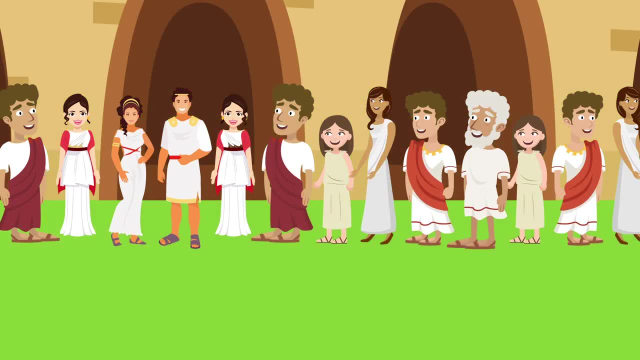 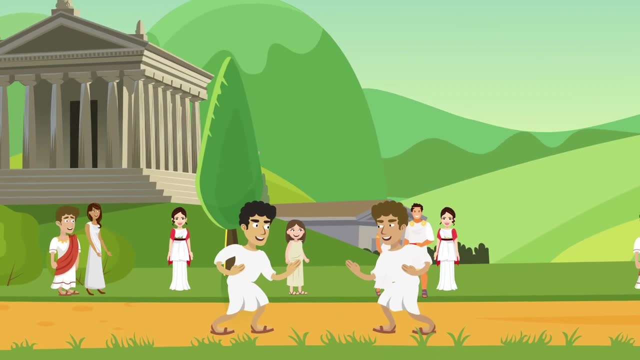 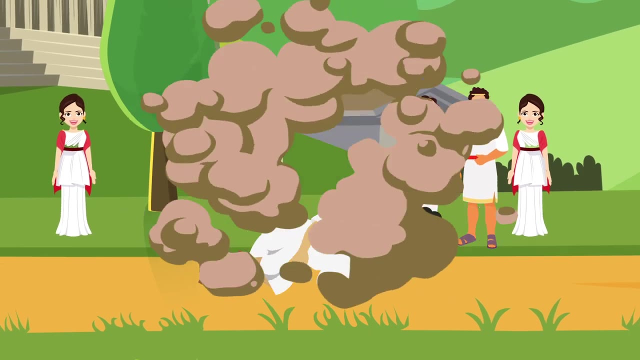 Empire, the popularity and importance of the Olympics diminished in favor of gladiatorial tournaments and other Roman competitions. Finally, in 393 CE, the Roman Emperor decided to officially abolish the Olympics, declaring it far too non-religious for their newly Christian empire. Just like that, the mighty Olympic Games were gone for good. 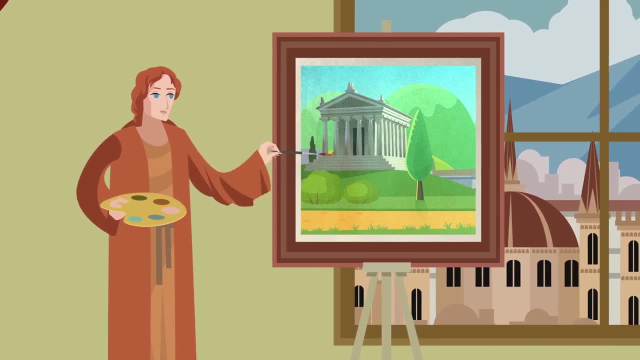 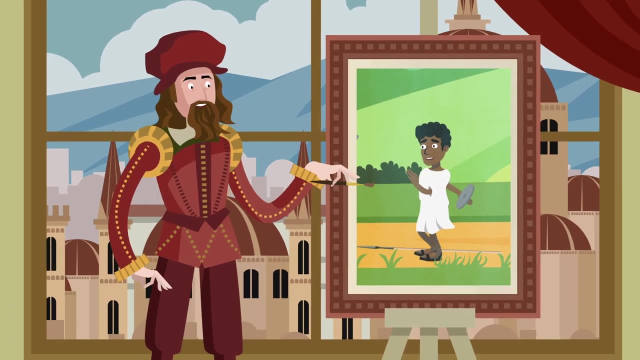 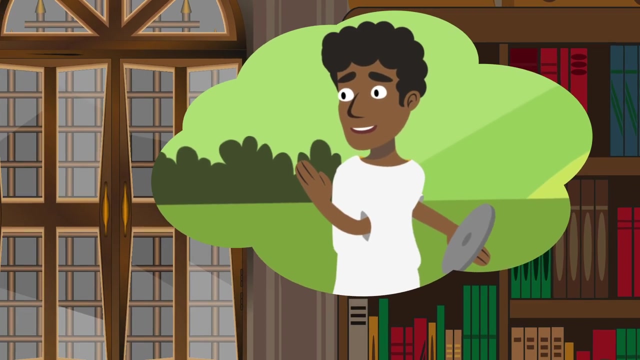 Or so it seemed. Around the time of the Renaissance, people began to get interested in ancient Greek culture. It became a major influence in art and got people thinking about all their different customs, including the Olympics. In 1892, the ball truly got rolling when a French historian 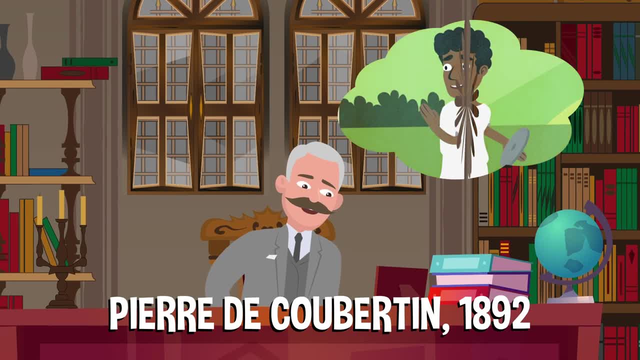 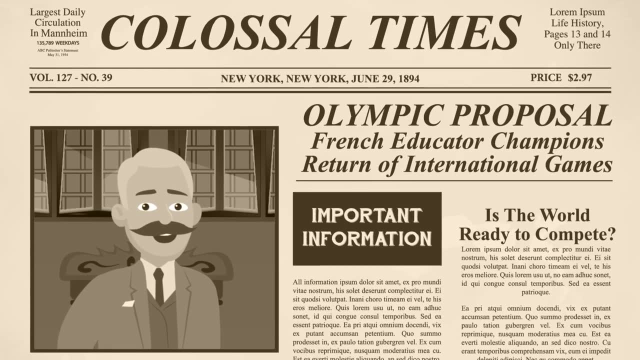 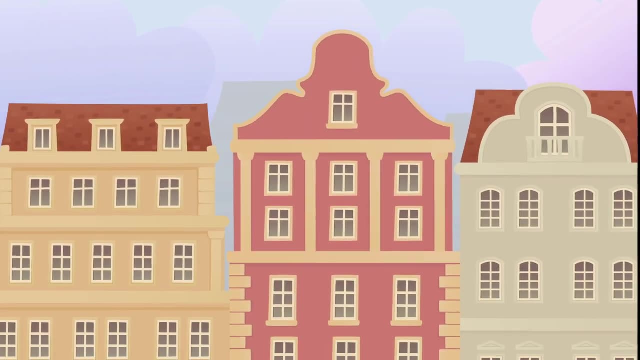 and teacher named Pierre de Coubertin made a serious proposal to revive the Olympic Games as a modern international competition every four years, bringing glory to the winners and their home countries. Two years later, Pierre's idea was approved and the modern Olympics finally got the go-ahead to start planning. 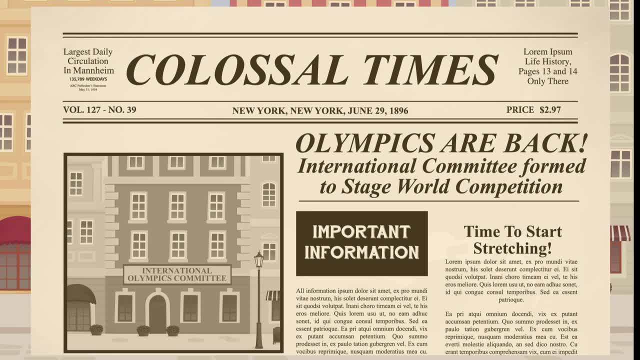 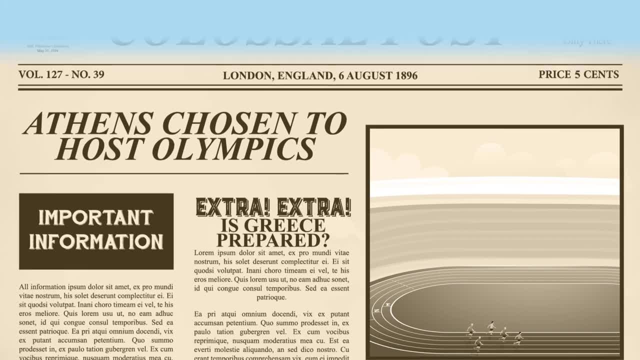 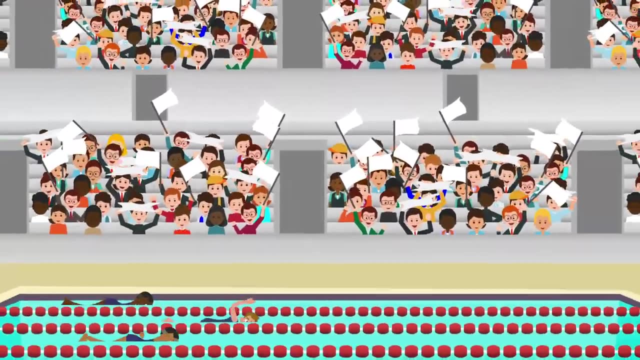 The International Olympic Committee was formed and the first games were scheduled for 1896. in where else but Athens, the capital of Greece? By the 1924 Olympics in Paris, more than 3,000 people competed, including more than 100 women from 44 different countries.